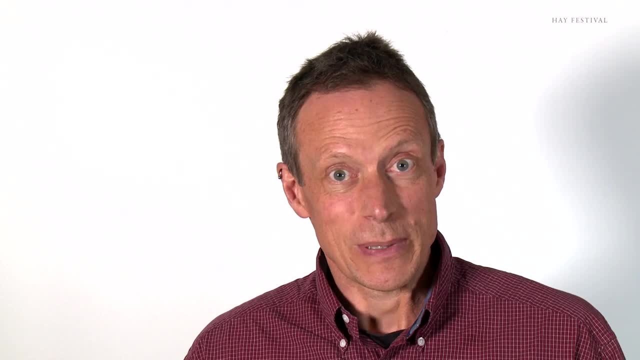 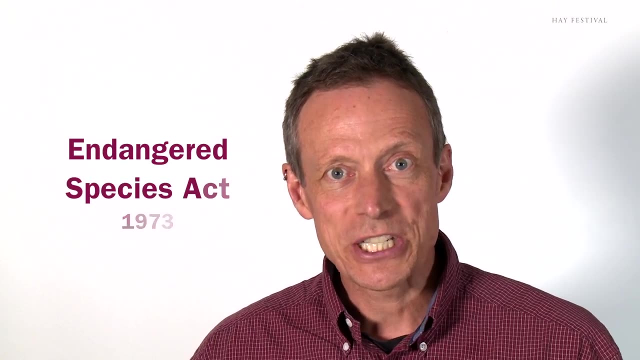 ultimately towards the whole planet. This has gone well. People have got excited about it. Some of the ideas, some of the words have made their way into legislation. In the United States, for example, there's an Endangered Species Act that specifically protects the 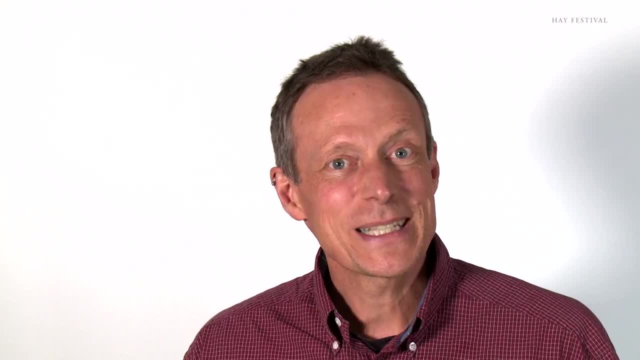 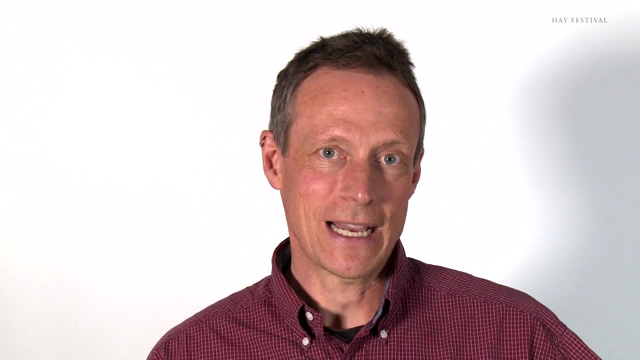 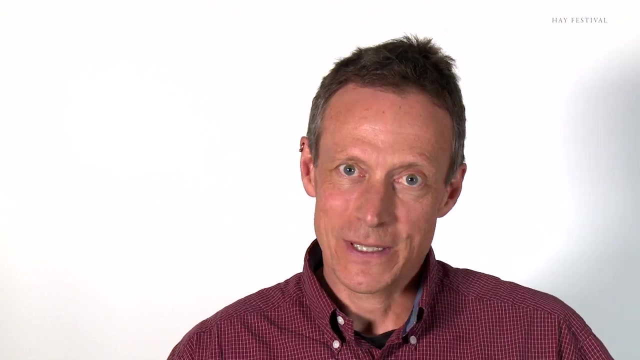 moral significance of endangered species. More recently, a problem has arisen. These things that have moral value must be separate from us. A tree is valuable because it is what it is as a tree, Or a wolf is valuable because it is what it is as a wolf. Those things are independent of humans. Now we live in a new 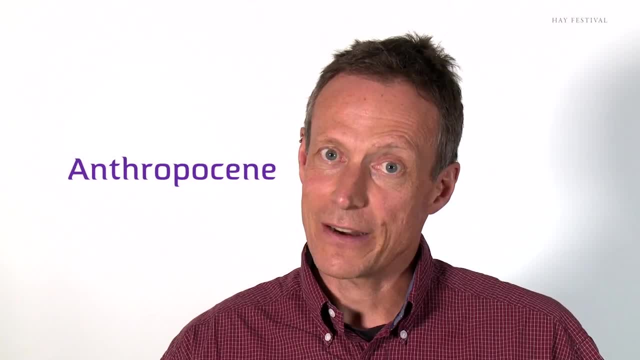 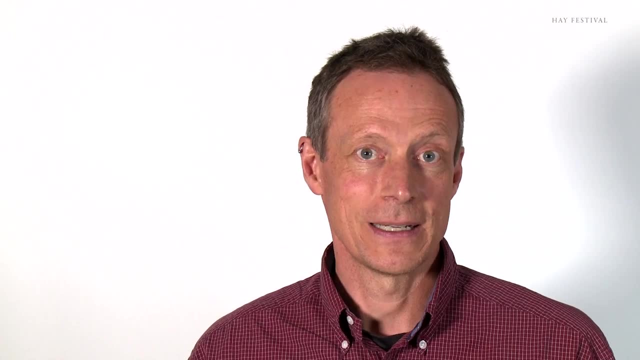 age, a new time, the Anthropocene, in which everything reflects some sort of human influence. So there's nothing out there in nature that is completely independent of us. This is a new world, And people have talked about the end of nature. So if nature has ended, what? 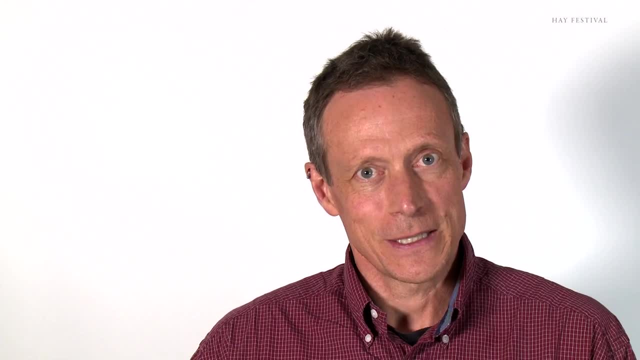 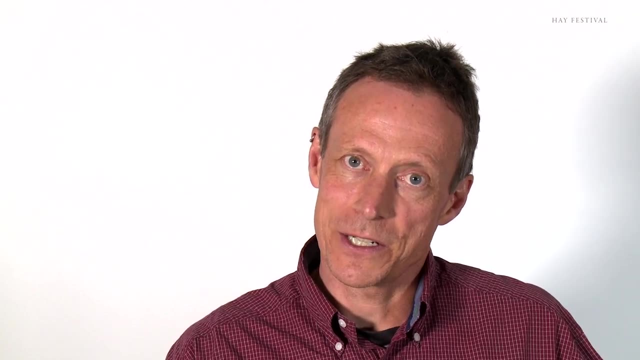 do we protect? What happens to environmental ethics? So it's a young field, but there's been a sea change in the last five or ten years, because we don't have nature anymore that is untouched or uninfluenced, And in fact it's worse than. 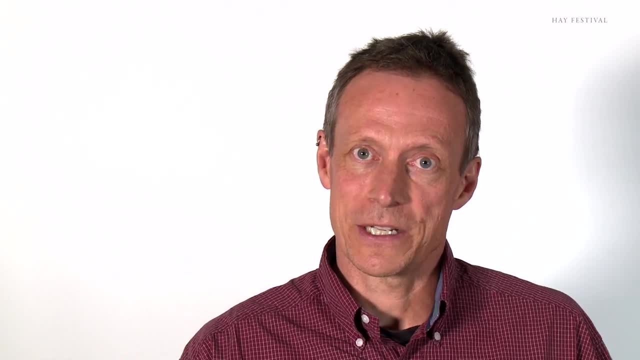 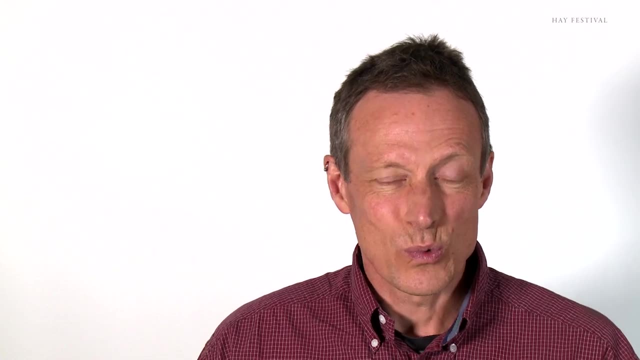 that It's not just that nature is now no longer untouched and uninfluenced. We have technologies at our fingertips that really get in under the surface of nature and recreate nature according to our own design. So the kinds of technologies I'm talking about are things like synthetic biology, where you 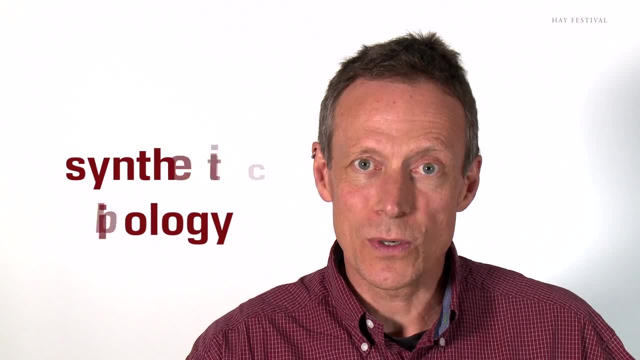 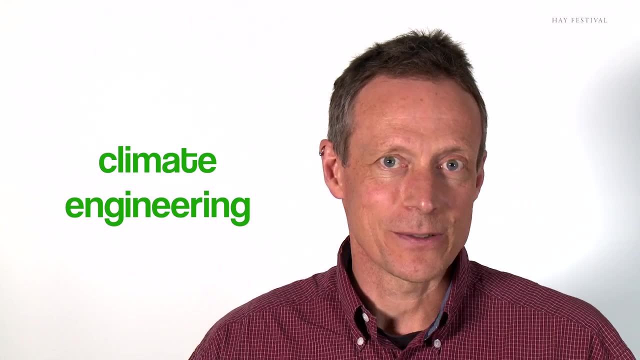 build genomes, you create life, you create new organisms and new species. Another technology would be climate engineering, where we interfere with the amount of energy that is arriving at us from the sun. What could be more fundamental than the amount of energy arriving on the? 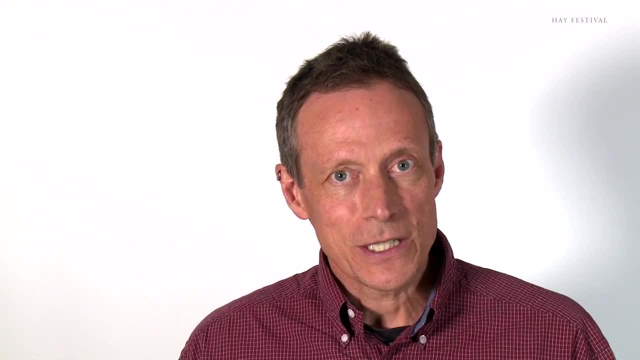 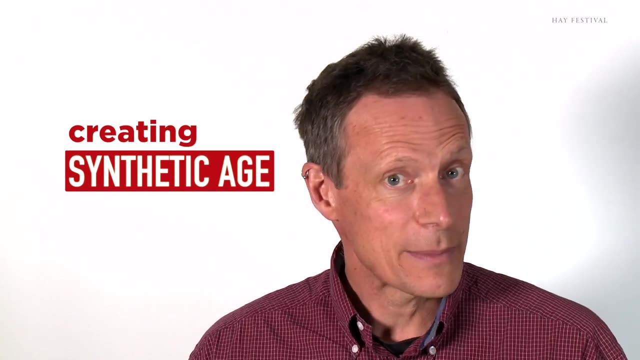 surface of the planet from the sun. So with these sorts of technologies, not only have we ended nature, we're beginning to create an entirely synthetic age, And environmental ethics now has to adjust to this idea of a synthetic age. So I'm going to give you a couple of examples. The first one is the idea of a synthetic age. 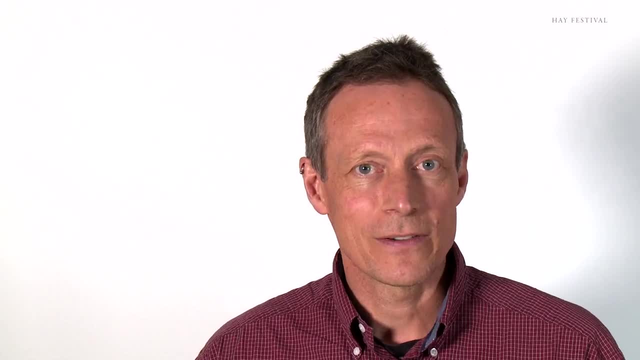 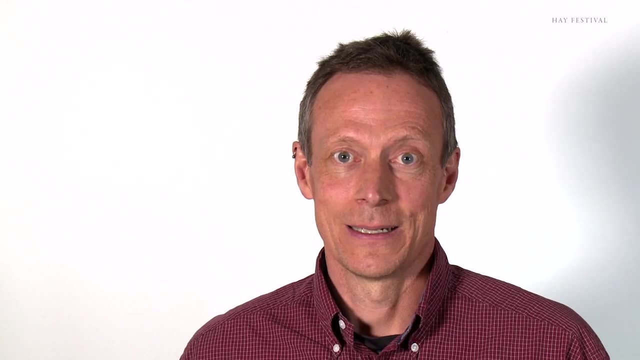 The second one is the idea of a synthetic age. The third one is the idea of a synthetic age. What sort of ethic would we have towards an organism that we created, Not an organism that was natural, but an organism that is entirely synthetic? So it's a new field. it's